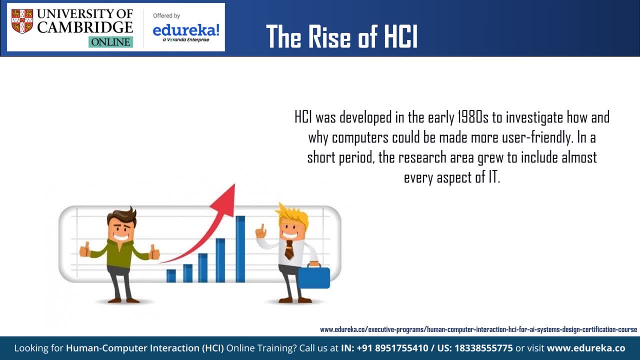 The use of computers has become much more widespread, making communication easier. The increasing recognition of the importance of user experience and user interface design has pushed HCI to the top. Companies are investing heavily in creating visually appealing and user-friendly interfaces. According to Sixfigurecom, the average salary for a Human Computer Interaction professional is approximately 21.7 lakhs per annum in India. 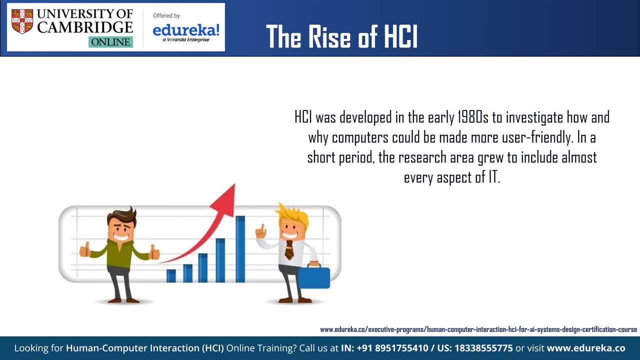 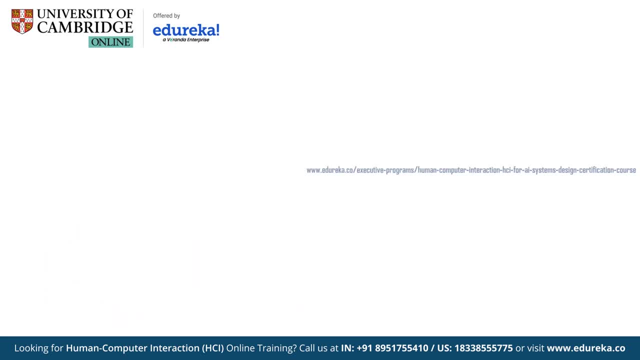 The estimated average salary for a Human Computer Interaction professional is approximately 21.7 lakhs per annum in India. The estimated average pay for a human-computer interaction professional is approximately $249,000 per annum in the United States. Now we will discuss the importance of HCI. 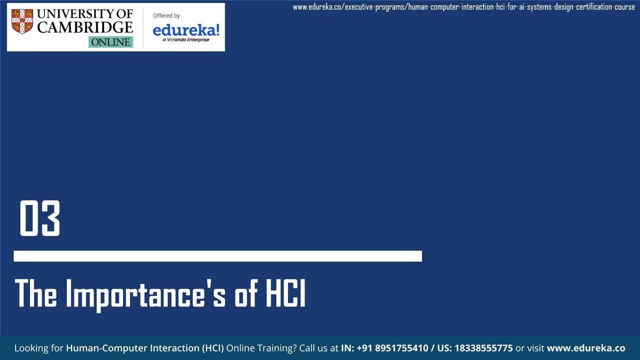 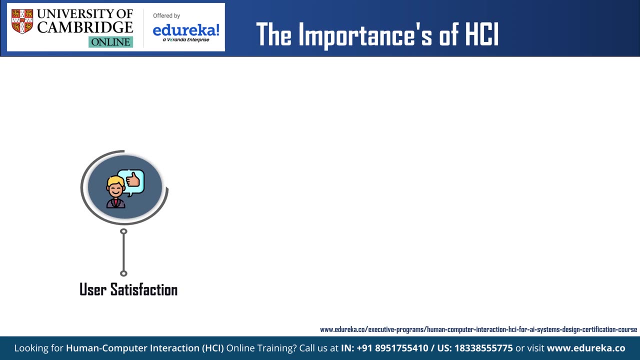 The potential of human-computer interaction to improve technological usability and design. making it more efficient and approachable is what makes it so important. Here are some primary reasons for the importance of HCI: User satisfaction. HCI ensures that technology is designed to meet the needs, preferences and expectations of its users. 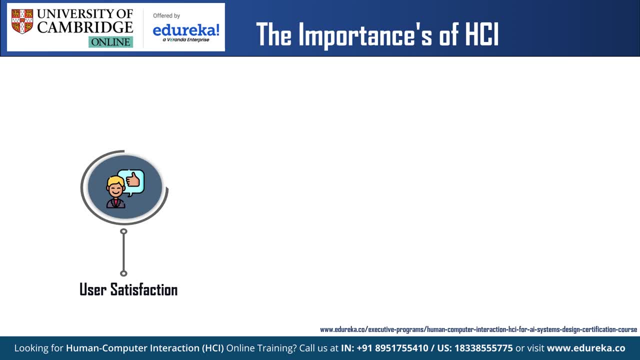 This results in products and systems that users enjoy interacting with Efficiency and productivity. Well-designed HCI can help users interact with technology more efficiently. Users can complete tasks more quickly and efficiently because of simple user interfaces and streamlined workflows. Error reduction: HCI design reduces the number. 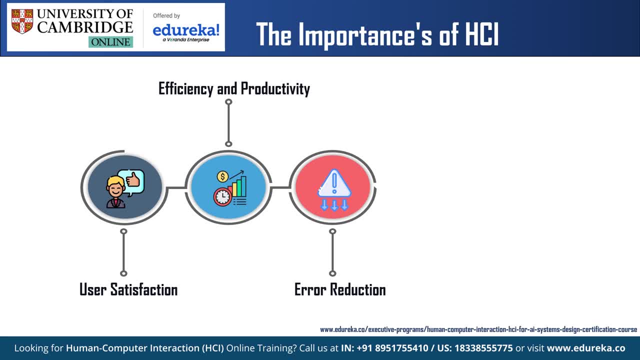 of user errors by providing clear feedback, simple navigation and user-friendly controls. This results in a more reliable and error-free user experience. Improving decision-making, Effective data visualization and information presentation, which are key aspects of HCI, assist users in making informed decisions. 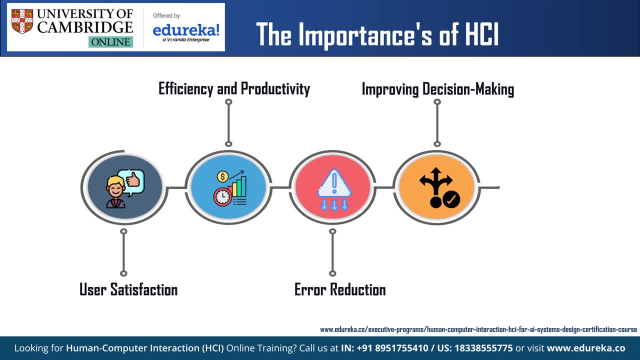 In fields such as data analytics and business intelligence. HCI is critical for transforming complex data into actionable insights. Innovation- Innovation HCI promotes innovation by challenging designers and developers to think creatively about how users interact with technology. This can result in breakthroughs in interface design and the creation of new types of interactions. 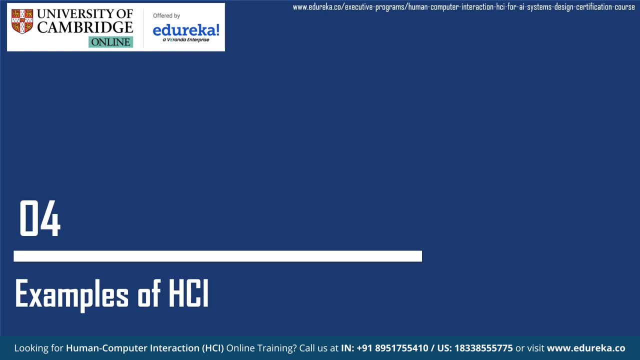 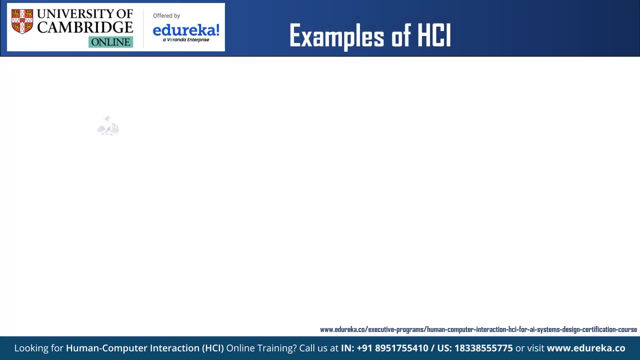 Now we will discuss the examples of HCI Human-computer interaction. examples are all around us on various devices and applications. Here are some common examples: Cloud computing. In the framework of cloud computing, human-computer interaction entails creating user interfaces and experiences for interacting with cloud services. 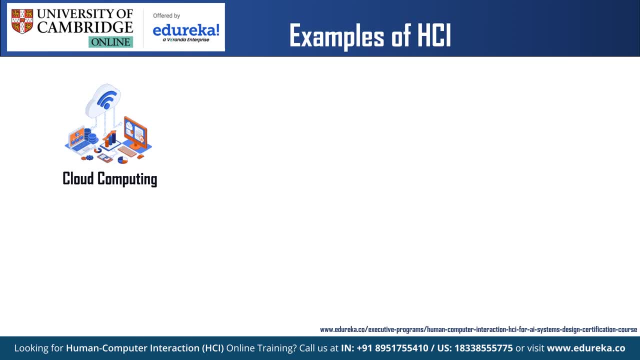 It focuses on creating user-friendly and efficient interfaces for tasks like resource supplies, monitoring and managing cloud resources. The goal is to improve user satisfaction, usability and overall experience in the cloud computing space. Free-touch sensing- Human-computer interaction and free-touch sensing- examines interaction techniques before direct touch contact. 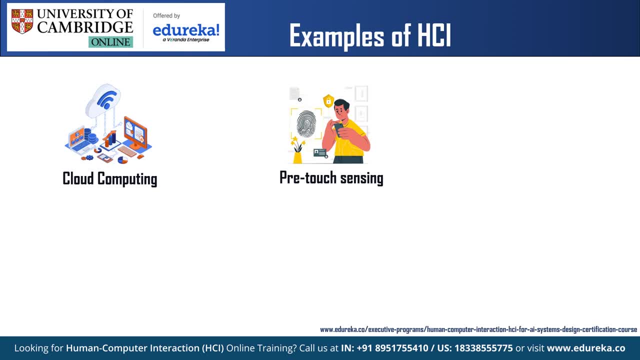 which frequently involves closeness or action. It aims to create interfaces that respond to user actions even before physical touch, thereby improving user experiences. Eye tracking, Real-time eye-tracking and human-computer interaction- uses technology to immediately record and analyze users' eye movements as they happen. 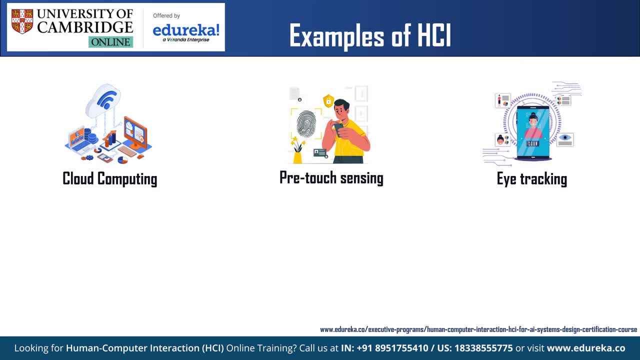 This allows for immediate feedback and flexible interactions, increasing the responsiveness and effectiveness of user interfaces. Chat, GPT: This is the focus of ChatGPT and human-computer interaction. This is the focus of ChatGPT and human-computer interaction is on designing and improving conversational interfaces. 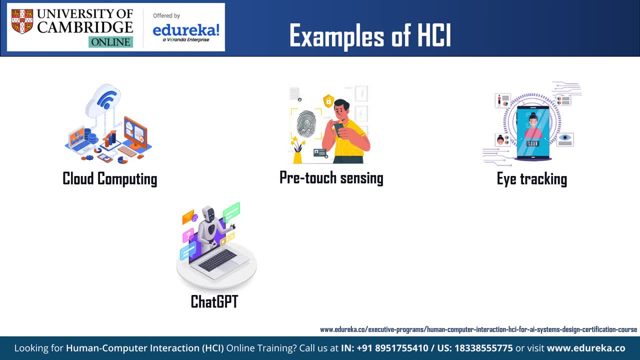 HCI principles are used to design user-friendly and natural interactions with chat CPT, taking into account natural language understanding, response consistency and overall user experience. Artificial Intelligence- HCI with AI involves including artificial intelligence in the design of human-computer interfaces. This collaboration aims to improve user experiences by integrating AI capabilities. 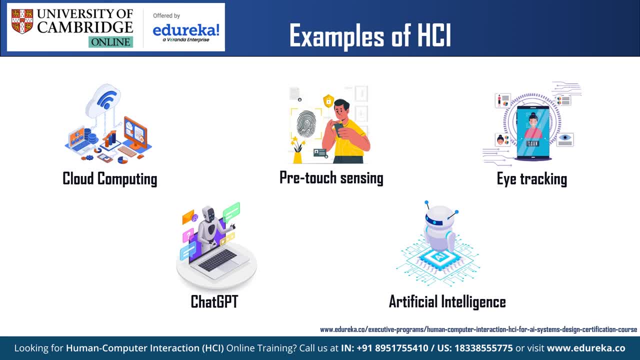 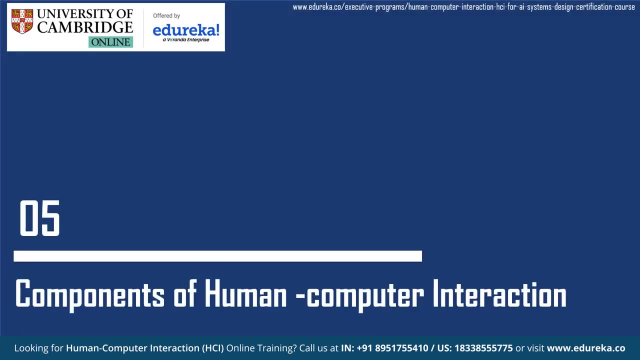 such as natural language processing and machine learning, into interactive systems. Now you have a clear picture of the examples of HCI. Let's move on to the components. Human-computer interaction includes a wide range of components that contribute to the design and usability of technological interfaces. 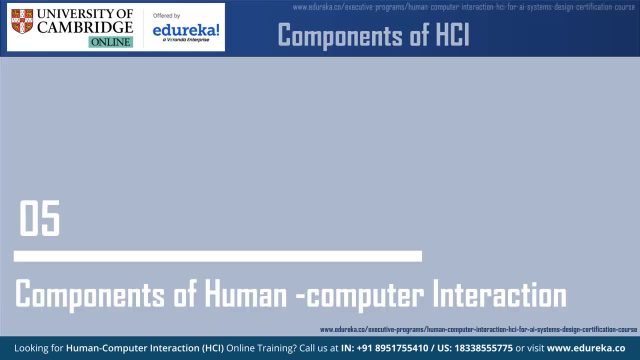 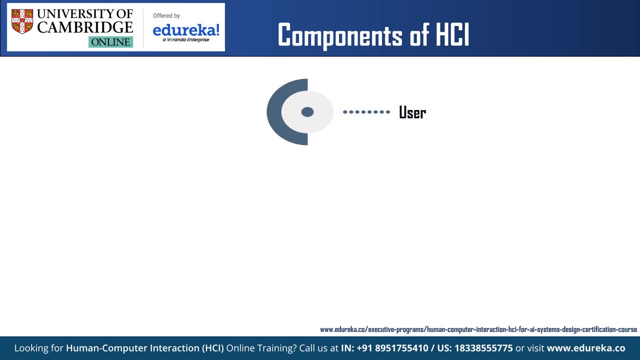 Here are some key components of human-computer interaction. User: The user is the person who interacts with the computer or technology. Understanding user characteristics, needs and preferences is critical. Interface- The interface is the point of interaction between users and the system. Interfaces may include graphical user interfaces, command-line interfaces, voice interfaces and others. 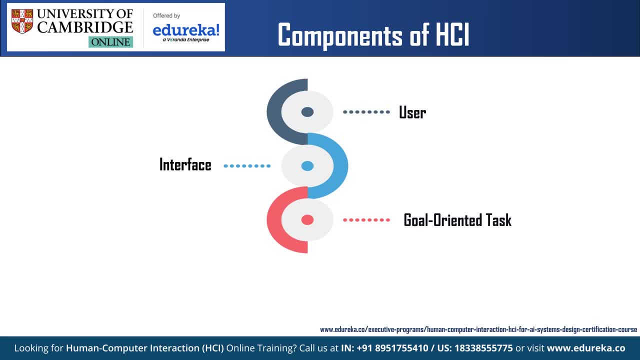 Goal-oriented tasks. When using a computer, the user always have an objective in mind. To accomplish this, the computer displays a digital representation of objects- Context. HCI involves not only improving user-computer communication, but also considering the environment. Now we will dive into the conclusion.